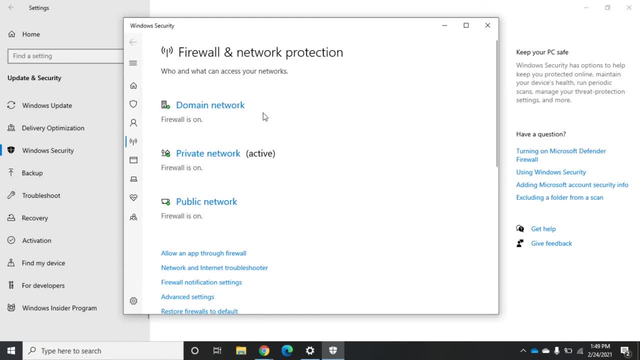 for more detailed information. So here is our firewall and network protection. You see, we have different domain pro or different network profiles: the domain network, the private network and the public network. And then this right here tells me that I'm currently on the private network profile. 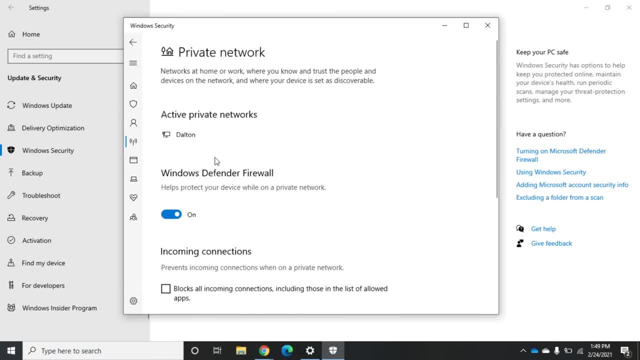 and currently the firewall is on. Now let me go ahead and click on that And I've got a couple of options here So I can turn off my firewall Now. I don't recommend doing this as a long-term solution, but if you need to turn off the firewall, 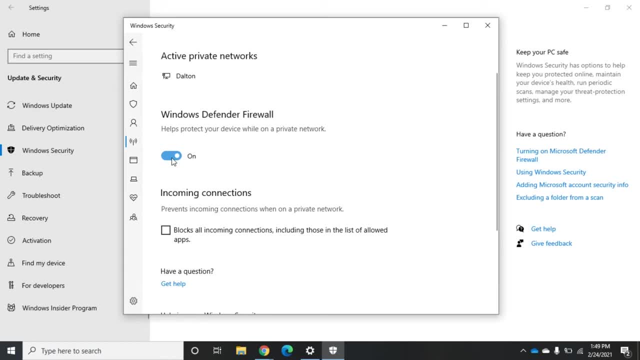 while you're troubleshooting an issue that actually can be useful. Something's not working. I'm trying. I'm having a network connectivity issue. Let me turn off my firewall, see if that fixes the problem. Now that does. I don't want to leave my firewall off, but now I know there's. 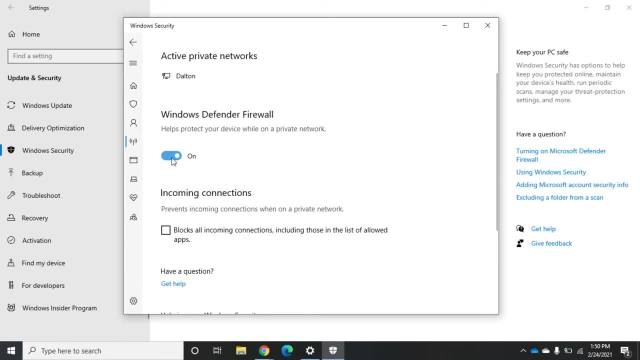 a firewall setting that I'm going to need to adjust. So I'm going to try to find that firewall setting so that I can bring my firewall back up But allow that particular application through the firewall. So this turns it off and then back on And it's now paranoid because I turned this firewall off. 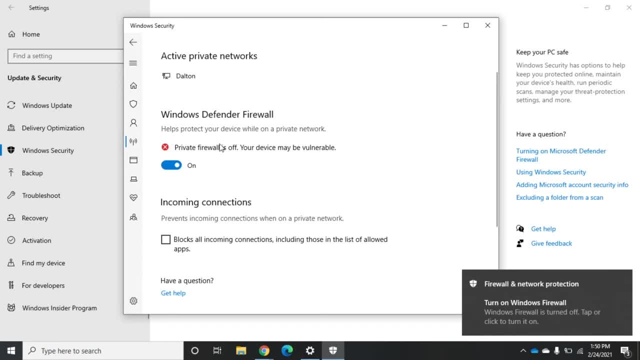 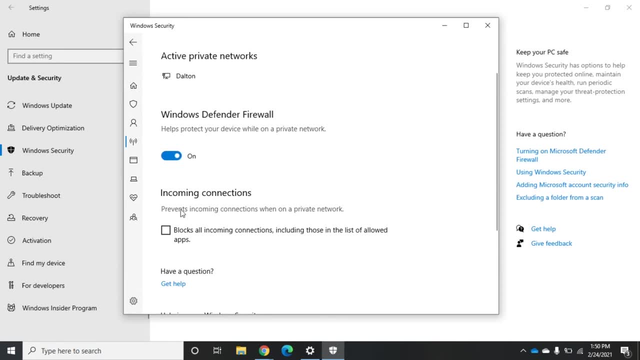 I'm going to turn this firewall back on. That'll make it happy again. Okay Now. so this is this on or off all or nothing thing. The other all or nothing thing is this one right here. So a firewall will control data coming into your computer and data going. 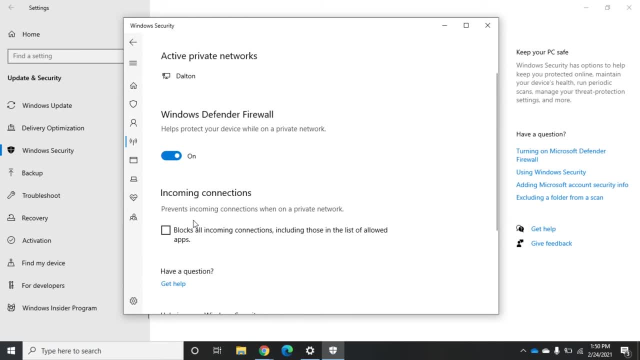 out from your computer. So this is a firewall that will control data coming into your computer and data going out from your computer And by default, Windows Firewall is going to allow some things going out, block most things coming in, unless they're specifically allowed. 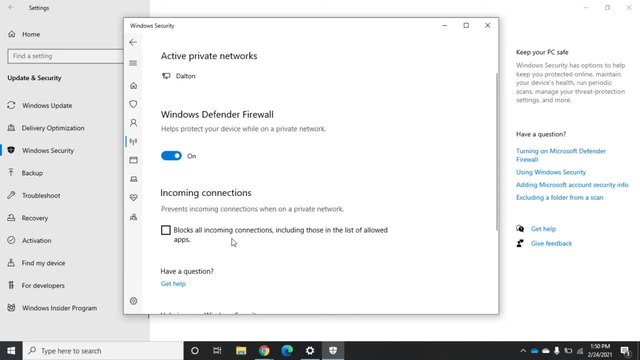 What this does is this blocks all incoming connections And again, this is going to be a temporary thing. This is not permanent, right? So I'm down at Starbucks and probably going to be on a public network, not a private network, but I'm down at a Starbucks and, for some reason, 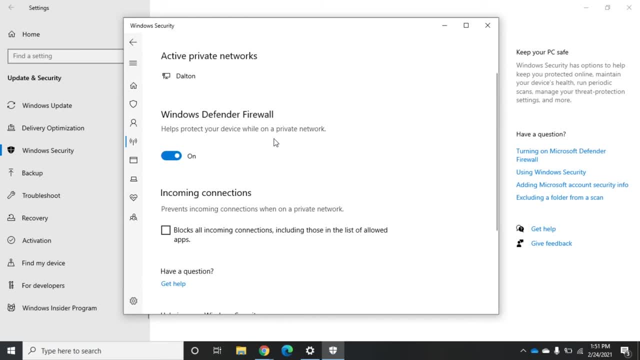 I just think you know what license number. You can't throw things in removed. you know Poker hasn't arrived, but you need to use this example in 1.3D. i'm on the network. i'm on the network, i'm surfing the internet. uh, i'm working on a document, but 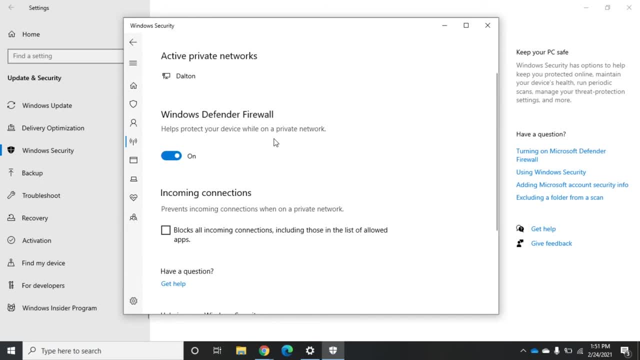 i really don't want any access to my computer across this network so i can come in here and say: just block all incoming connections, including those that would otherwise be allowed, and that's just gonna, you know, slam the door shut. so when we turn off windows defender, you know get rid of all. 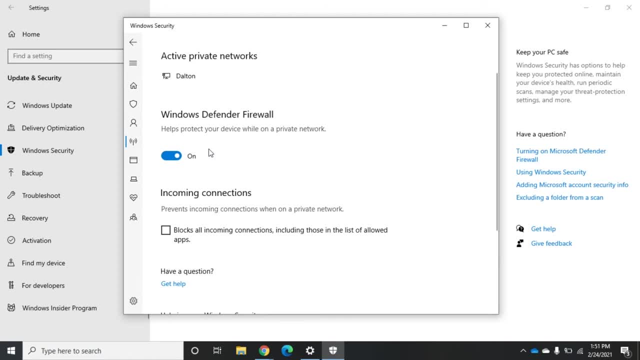 the locks on the doors, throw open the windows, knock down the walls, just let anybody come in. this is the exact opposite. go complete lockdown. okay, those are two all or nothing options and we can do that for any one of these three profiles so i can send my public network. i want to block. 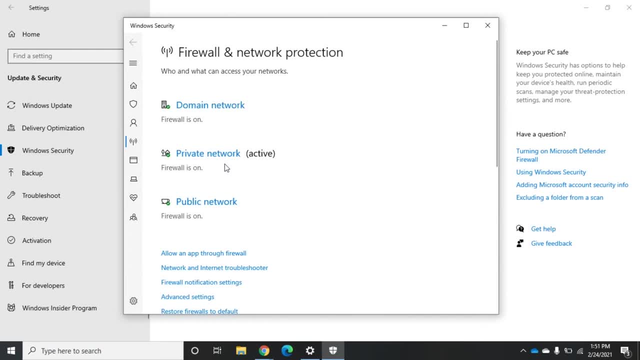 all incoming connections while still leaving incoming connections allowed on a private network that i trust a little bit better. all right now, those are all or nothing. most of the time we don't want all or nothing. most of the time we're going to want specific things, and that's here. allow an app through the. 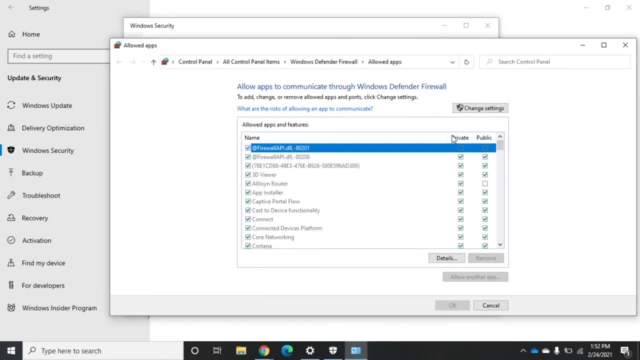 firewall. so let me bring this up and this is going to show a bunch of apps that are already allowed through my firewall, and so you'll see the list of apps here, and a bunch of these are going to be microsoft apps, but there are some of them that are not going to be microsoft apps, like i have. 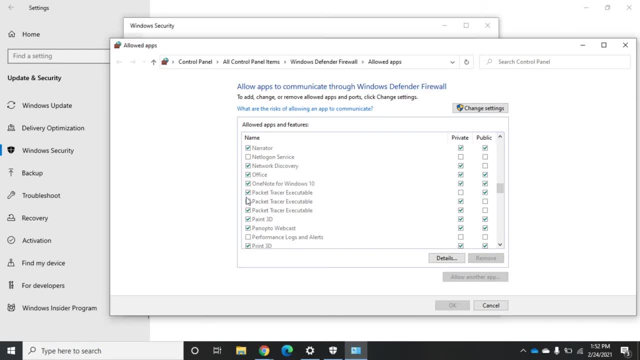 packet tracer installed on my system and so packet tracer created a rule for the firewall and it's going to say, hey, go ahead and allow this. and i didn't do that right when i installed the software, the software did that for me. so that actually makes this easier to work with. but if for some, 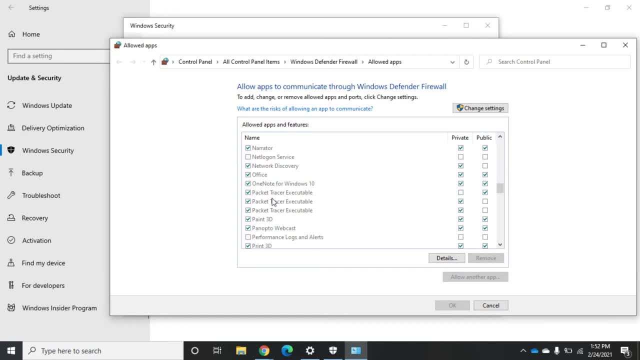 reason, i decide that there's an app that i don't want access to after all, then i can come in here and i can change that. so we'll do that by going to change settings. and let's look at this one right here: paint 3d. so paint 3d is currently allowed for both the private and the public network. 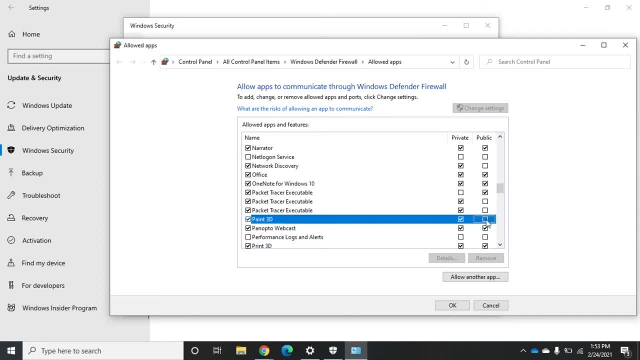 change which networks it's allowed on. i can just click that and uncheck or check those boxes. if i want to turn it off entirely, i check the box over here- pretty straightforward if i don't see the app in here that i want. so let's say i'm having a problem with a particular application connecting. 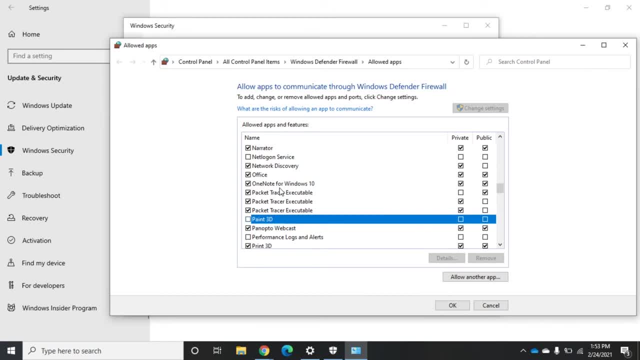 through my network. i've proven that because i turned off the firewall and it worked fine. turned the firewall back on, it stopped working. okay, so that told me where the problem was. so now what i can do is i can come in and i can go to my network, and i can go to my network and i can go to my 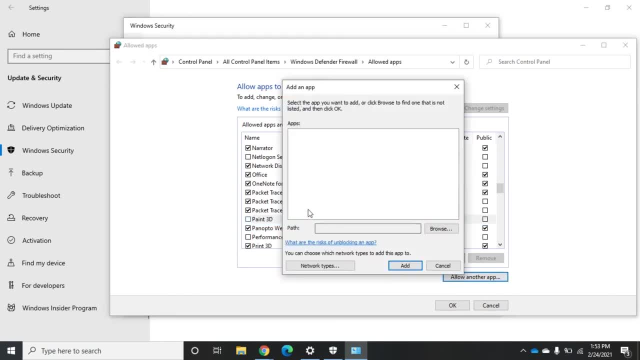 application and add another app, so i allow my other app. i browse to wherever it is blah blah. i find my app. i'm already in packet tracer. go to click that, just for the fun of it. so i'm a packet tracer. and then i'm going to choose network types- public or private network- and then go and cancel. 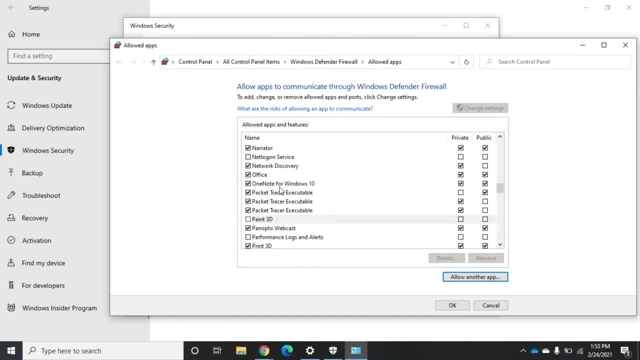 that, because i don't need it. that will add that executable to this particular firewall rules to allow them out either public or private networks. so this is the easy way to manage it. this is not the detailed way. this it does it based on application, not on specific port number. now, if we want it on specific port number- and i want more- 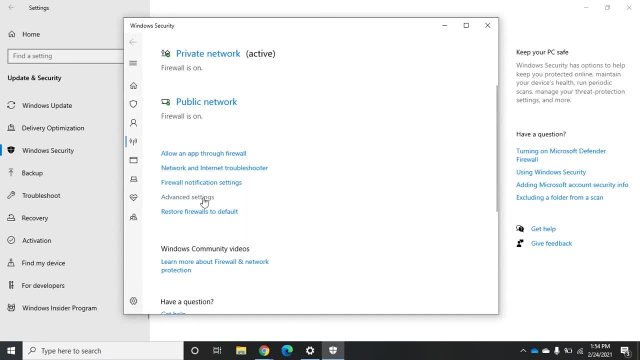 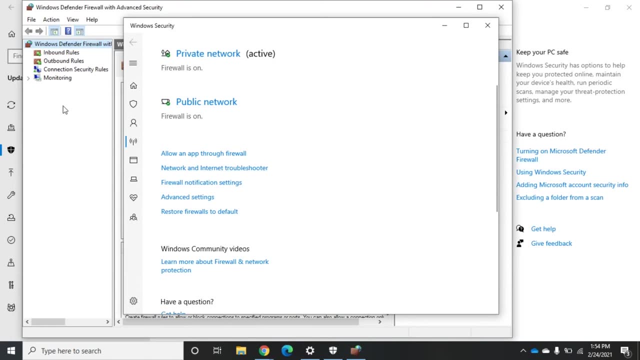 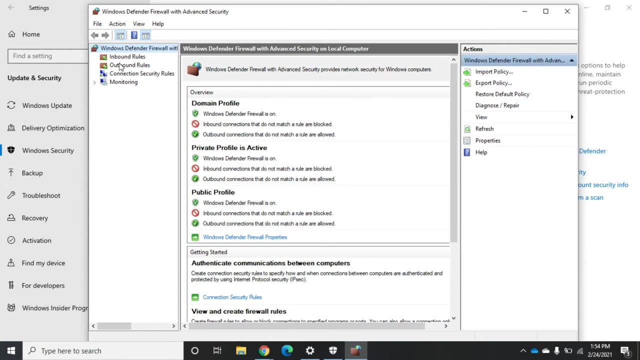 detailed settings. that's where i go to my advanced settings. so i'm going to click my advanced settings and here is my windows firewall with advanced security. now, over here i've got different types of rules: inbound rules, outbound rules, connection security rules. here's my little overview and specific actions i can take. so for each of these profiles, the windows defender. 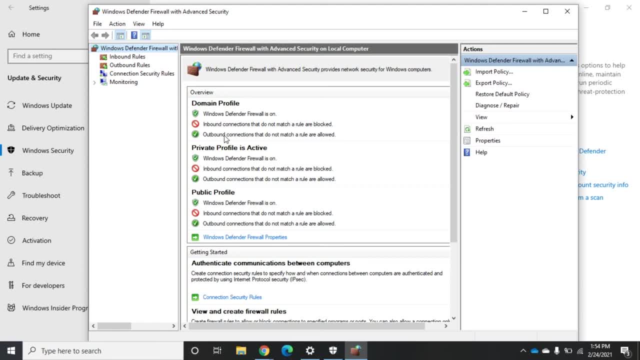 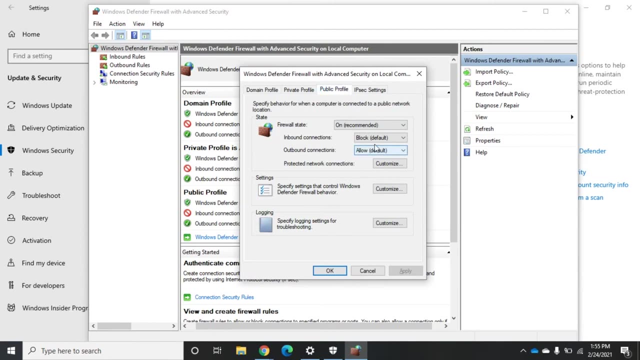 firewall is on. inbound connections do not match rule are blocked. outbound connections do not match rule are allowed. now, obviously, i can change these however i want as well, by going to windows defender firewall properties. and so then, for, let me go to my public profile, and from my public profile i can. 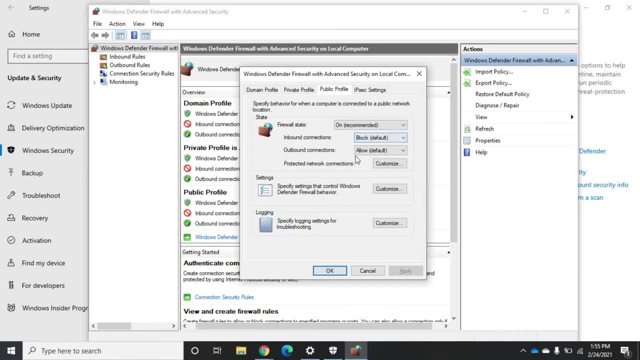 say, firewall status on inbound connections blocked by default, outbound connections. i'm going to block outbound connections now. obviously i don't want to actually do that, but if i did want to, you know, completely block any access to this uh in or out of this computer. well, i'm on that public network. 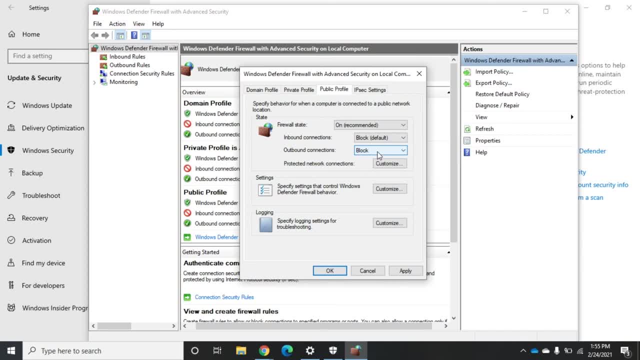 that would be a way to do it. this is going to block my outbound connections, so nothing originating on my computer going out will work. and then on my inbound connections, i can block default. block all connections or allow all connections. allow all connections, no security. block all connections. at this point i would go into complete isolation mode you're going to apply. 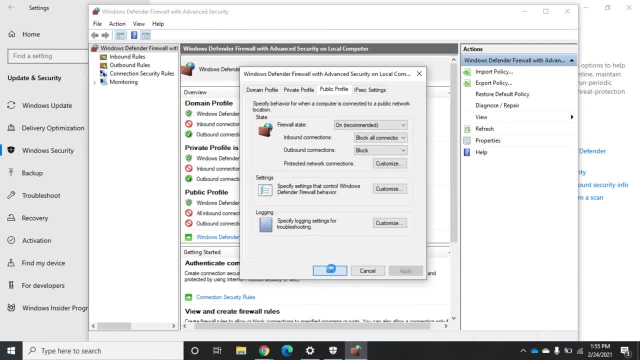 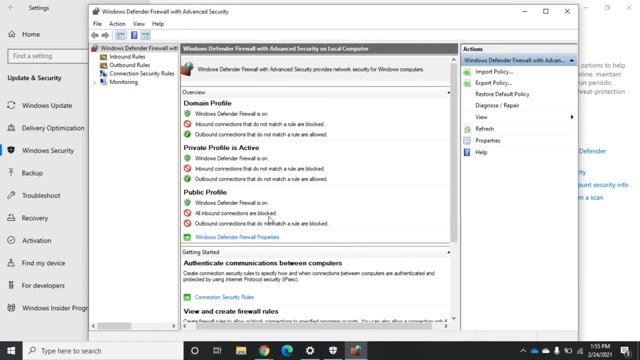 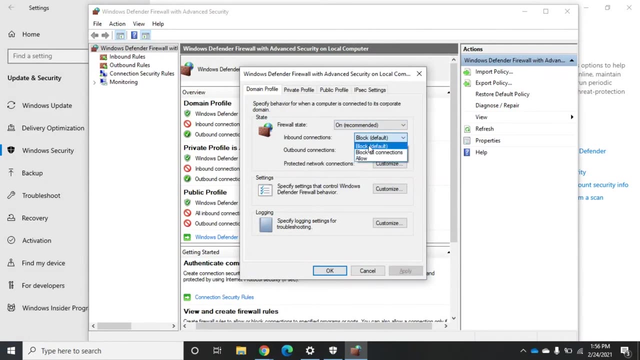 that because i'm not on this network anyway and we'll see right here. windows defender firewall is on and we are blocking everything. so if i ever switch my network profile to public, it's my firewall goes into complete lockdown. so let me go to do, do, do, do, get my right profile here again to reset that. 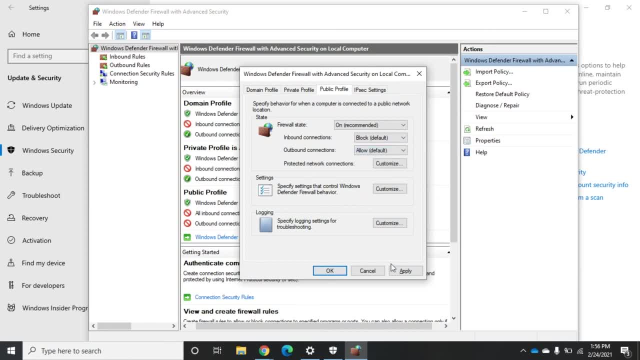 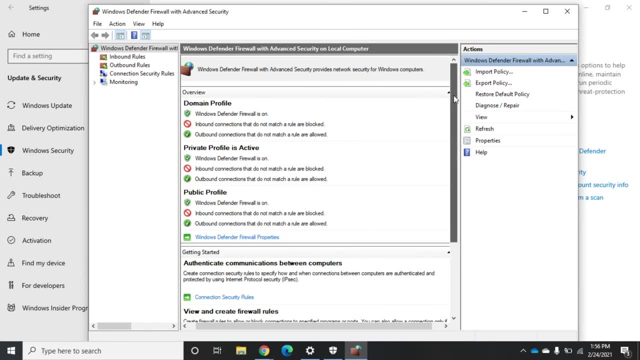 okay, so those are very, very similar to some of the things we were looking at when we were looking at the basic setup view and create firewall rules. all right, let's take a look at our inbound and outbound rules. inbound rules: impact traffic coming in. outbound rules: impact traffic going out. let's 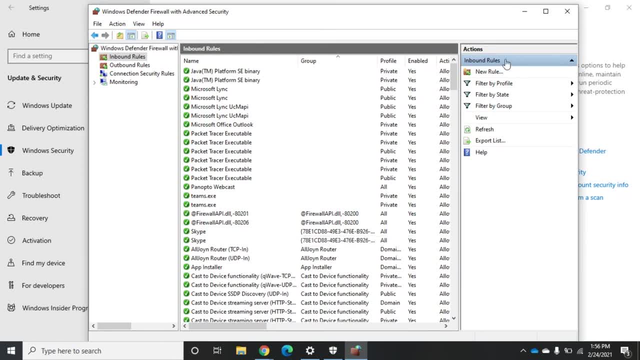 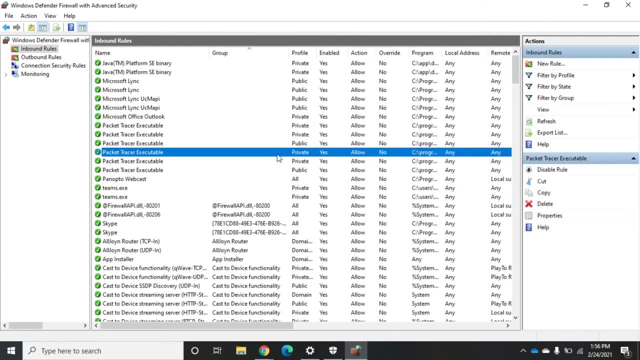 start with inbound rules. here are all of our inbound and outbound rules, and we're going to go ahead and maximize this. give us a little more real estate here. so let's take a look at this packet tracer: executable. what profile we're looking at is enabled. what action does it take- block or allow? 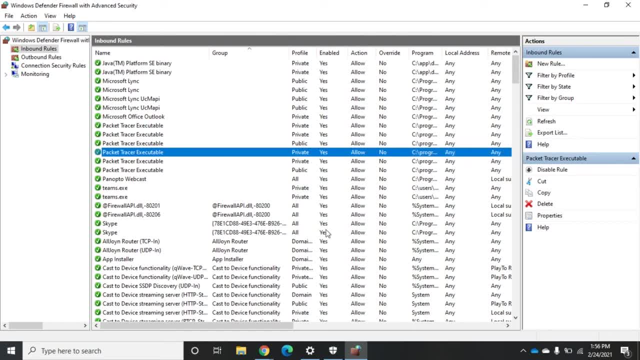 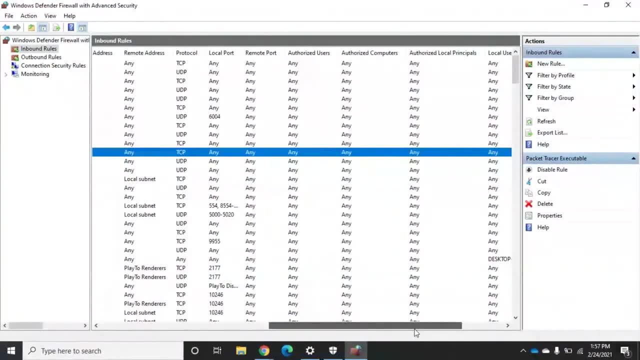 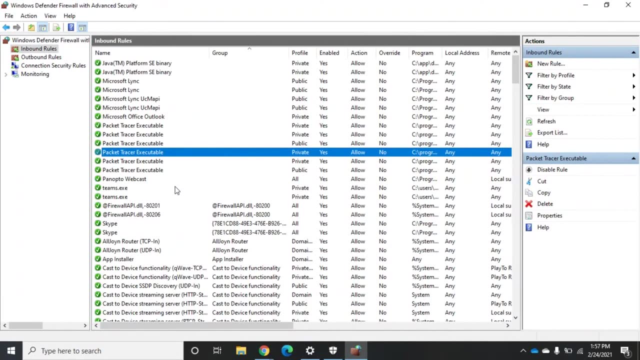 what program does it entail? what's the local address, what's the remote address? and then, as we scroll over, what protocol, what port number, what remote port? local and remote port number- are there any authorized users or computers? or well, as you can tell, these can get fairly detailed. maybe the best way to look at this is going to be to go and create a new rule. 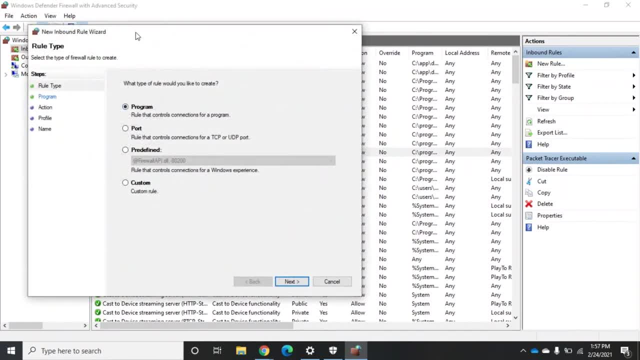 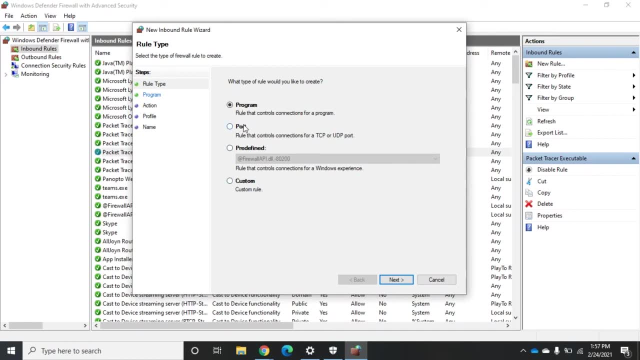 so i'm going to come over and click new, new rule, and i can do this based on a particular program, a particular port number, a predefined rule or a custom rule. let me start with a port number. let's say i want to allow port 25 for smtp connections in only be relevant if i'm running a mail server. 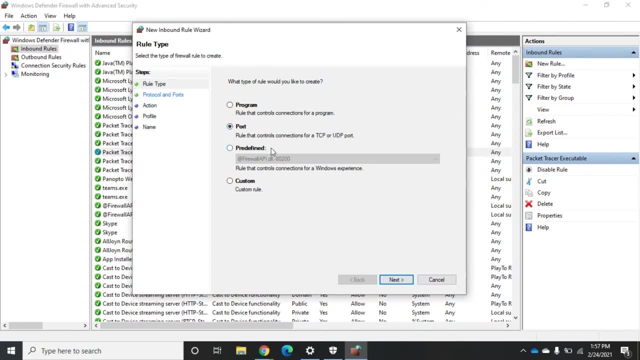 i'm not, but we're not going to save the rule anyway, so let's click on. we're going to do a port rule and we're going to go next. is this going to be a tcp or udp port? as you can tell right away. in order to do this, you need to know which port numbers you're working with, what protocols you're. 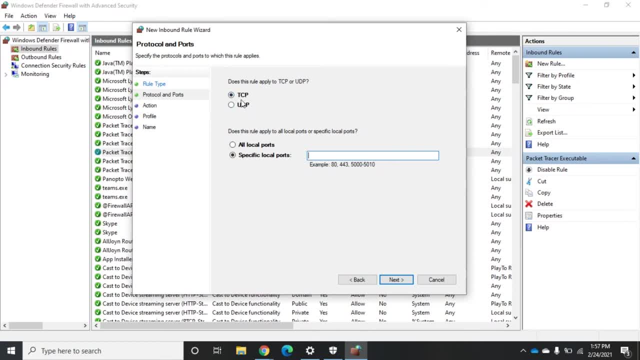 working with. so this for a mail server is going to be tcp port 25.. so i'm going to specify port 25. i really don't want to specify all local ports. that's opening things up way too much. i notice i can set up more than one port here. you see there examples separated by commas or a dash for a range. 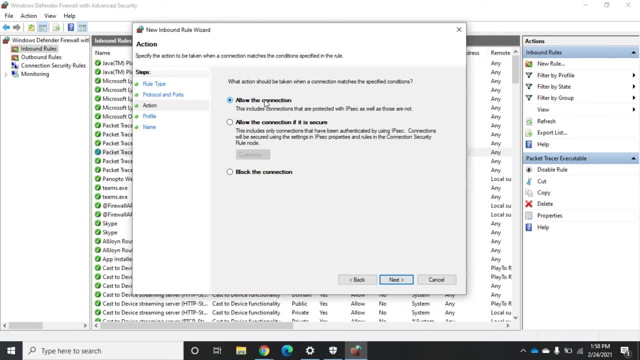 i'm going to do port at 25 and then i have three options. so i can allow the connection- allow only if it's secure- so these are ip set connections- or i can block the connection. now blocking connections is kind of weird. normally you don't need to block connections, you just don't allow it if it's. 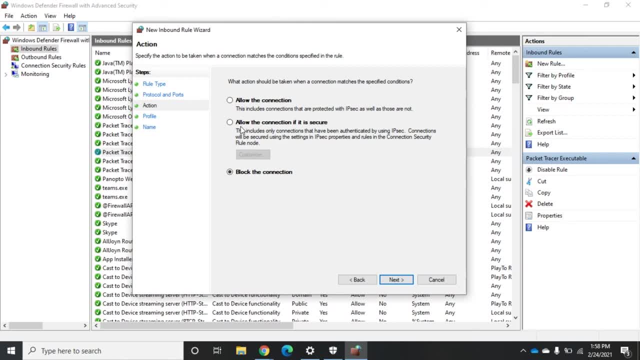 not allowed, it's blocked. but sometimes you'll have another rule somewhere that's allowing something and this particular type of traffic is part of what's being allowed, but you really don't want this. in that case you might need to use a block rule, but your better option is to only create. 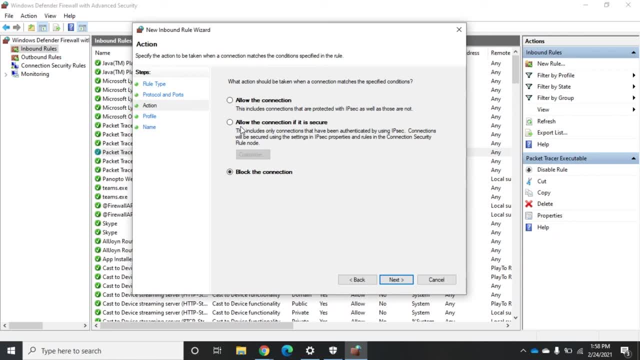 rules for the data that you want allowed and just let everything else be automatically blocked. so i'm going to allow this because i'm going to be running a local mail server. and then, what profile do these apply to? domain private, public, and i'm only going to run this. 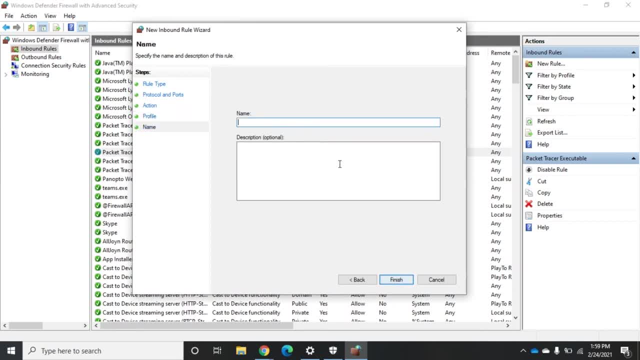 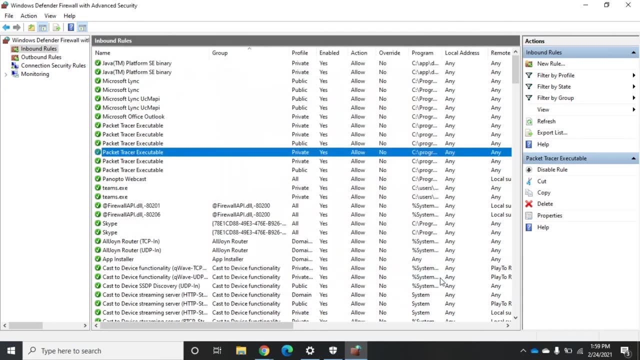 when i'm on a domain network and click next, and then i'm going to set the name in the description for the rule and click finish and that'll create the rule for me. i'm going to go and cancel that because i don't want to actually. 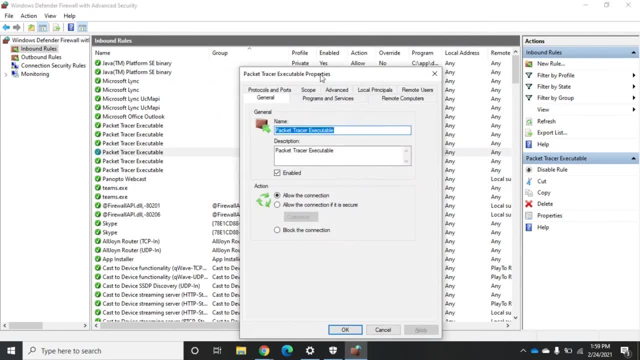 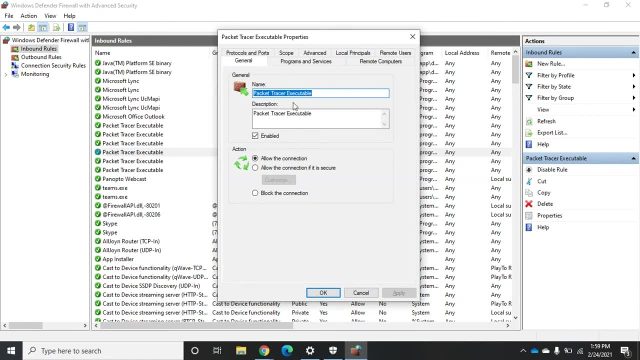 do that. let's open up another rule here so that we can look at once we get it created. this is going to be all the details for it. so this is a rule for packet tracer, so we got the name of it, the description, whether it's enabled or not, what it does. it allows, the connection. we can look at the. 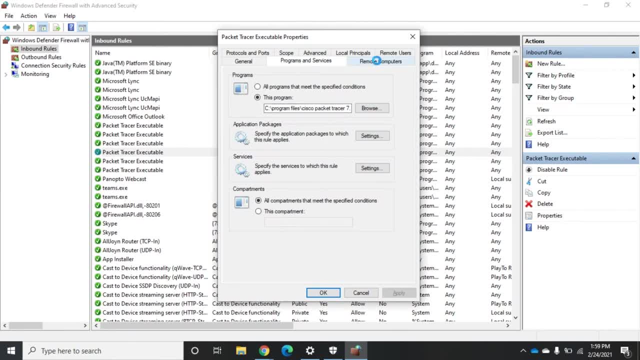 programs and services that are allowed to use this, and then any remote computers. are there only specific computers that we want? are we going to make exceptions? so by default it's going to allow anything. but i can say you know what, only allow these specific computers or skip this rule for these specific computers. so i want packet tracer. 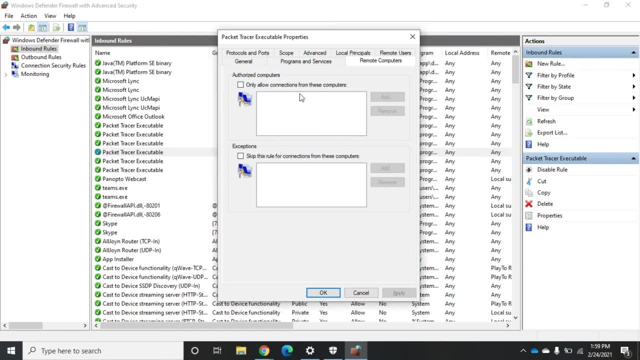 to work with everybody except, and then i can specify my specific exceptions. you can also identify specific protocols and ports. so what if i don't want packet tracer to use all ports? well, i can specify specific ports that would be allowed to use. obviously, i'd have to modify the rule, but, um, you see here where we can set it. um, we can set the.